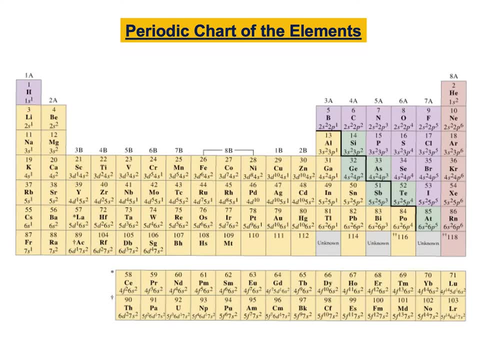 Dear students, welcome and thank you for tuning in. We are continuing our discussion about ceramics as part of the material science class and the biomaterials class. Here we're going to look at where can we find the elements that make ceramics in the periodic table and talk a little bit more. 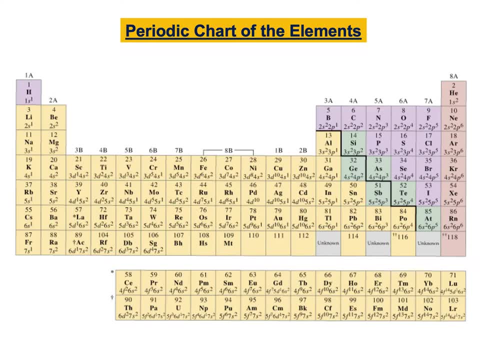 about the properties of metals and non-metallic elements of the periodic table and how do they relate to ceramics and the bonding in ceramics. This is a picture of the periodic table. We are all familiar with it. We would like to distinct two regions in this periodic table. This region 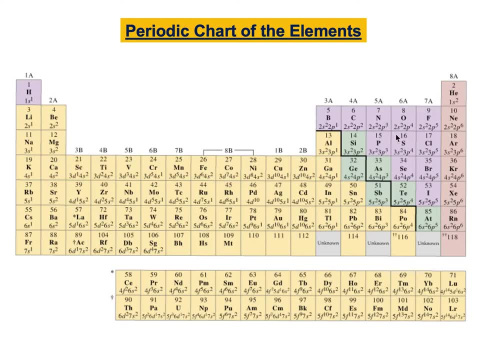 in the yellowish color and this region here in the purple color. So this region, here are the regions that represent metals and most of the elements on the periodic table are metal. I think there are 88 of them are metals. This purple region is the non-metallic elements: Ceramics. 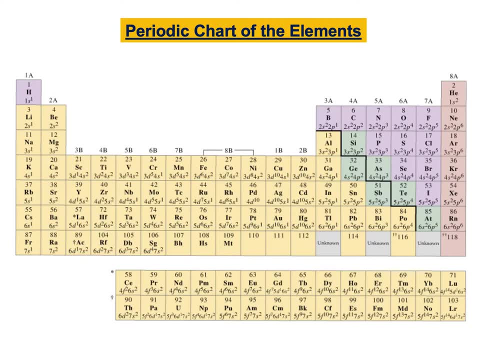 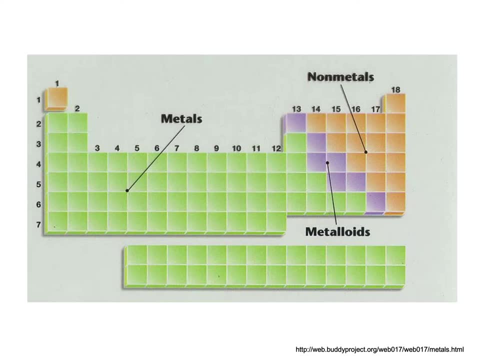 are made of non-metallic inorganic elements and they can be combined between the two, metallic and non-metallic. This is another schematic or representation of the elements in the periodic table. Everything in green is metallic and everything is on orange are non-metallic elements, and there are some, you know, in the middle, metalloids- that's what we call them. 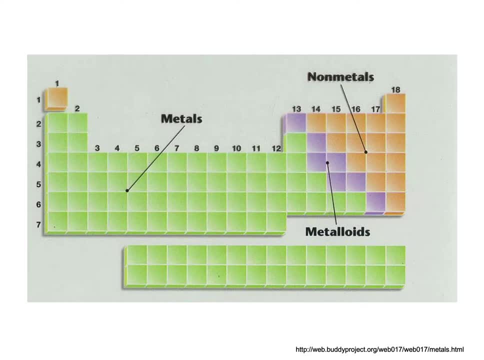 Now let's go to look into what are the characteristics of the elements here, the green elements, what are the metals and what are the characteristics of the non-metallic elements. So a quick review: most elements are metals: 88 elements in the periodic table to the left of the. 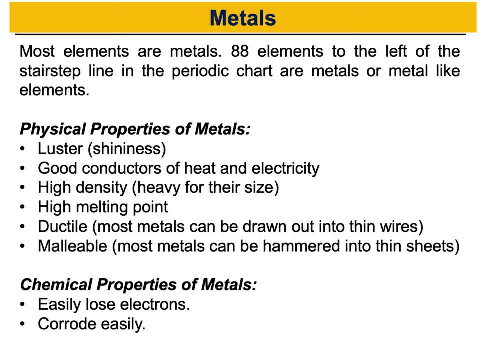 right. The first step line are metals or metal-like elements. So what are their physical properties? You can read them and you can see. they're shiny, they reflect light, They're good conductors, They have high density, high melting point. They're ductile. So you can. 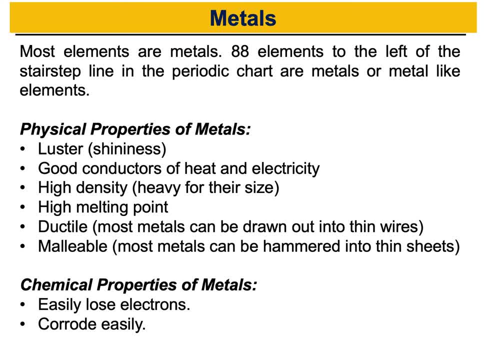 shape them easily into the shape or the form that you want to do, and this is one of the applications. This is one of the reasons why we like metals in engineering: because we can shape them the way we want. Malevolent metals are metal-like elements, So they have a certain density. They're 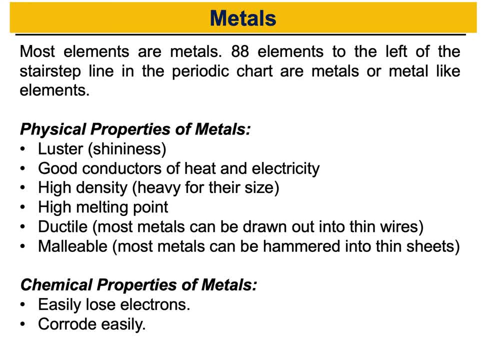 not completely metallic. They're not completely metallic. They're not completely metallic, So they have. Also, most metal can be hammered into thin sheets, so it comes down to ductility. So that's one of the reasons why metals are widely used in engineering. 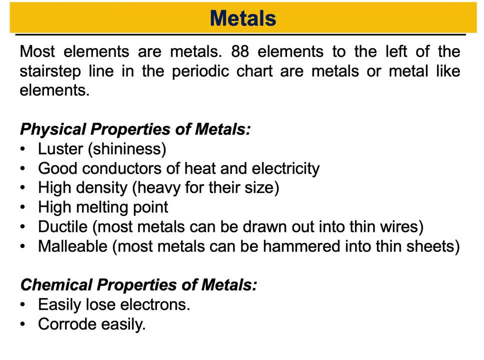 Also this is physical properties of metals, The chemical properties of metals. they easily lose electrons when they are surrounded, let's say under certain conditions, and they corrode easily. And we will discuss corrosion later on And corrosion it is an electrochemical reaction. 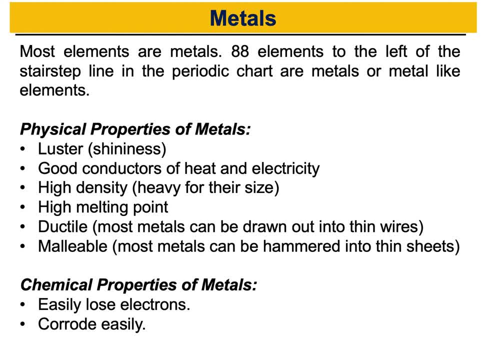 So we have chemical reaction and there is an electrical unit that is formed to result in corrosion, And we're going to discuss that in detail. So those are the characteristics of metals And for us as engineers it's important to understand them because degradation, because of the chemical property in losing electrons and corrosion, is a determinant factor in engineering applications. 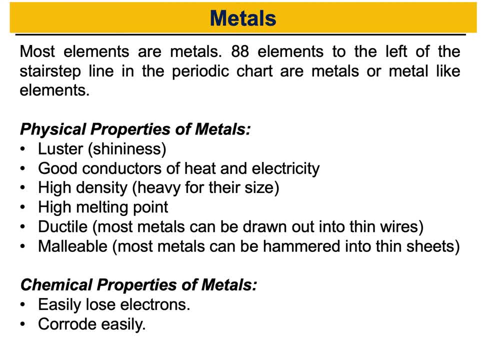 You don't want to have corrosion. You don't want to have corrosion or degradation of your components if you are building in to withstand loads for long periods of time. So, and also it's conducting energy and heat and high density. So all of these things. 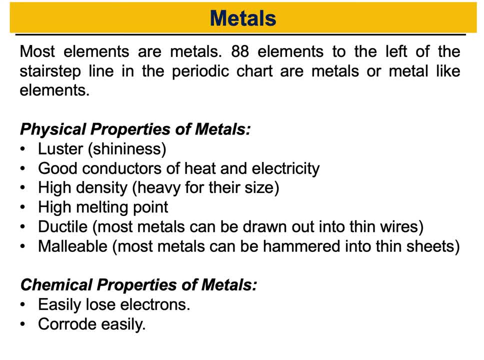 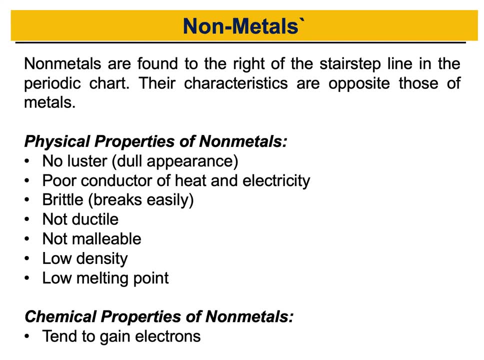 But you need to balance. what do you need for the application that you're looking for? Ductility is important and malleability perfect. However, corrosion is a challenge in metals. That's why we look at non-metallic elements, So they are found to the right of this table. 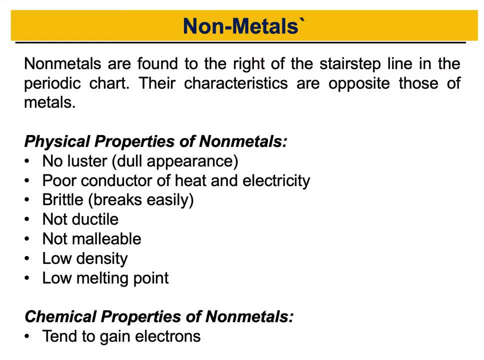 They are found to the left of this table. So, as we mentioned before, they're here. and those elements characteristics are opposite to those of metals, so they're dull, they're poor conductors, they're brittle, very poor ductility and malleability, low density and low melting points. 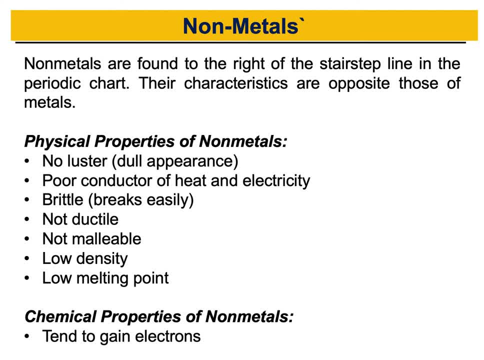 Now here's what happened. Also, they tend to gain electrons and they don't corrode, So it's opposite to metals. That's why they can interact, Interact with metals and create elements. you know different elements that are elements that are made of metal: metals and non-metallic elements. 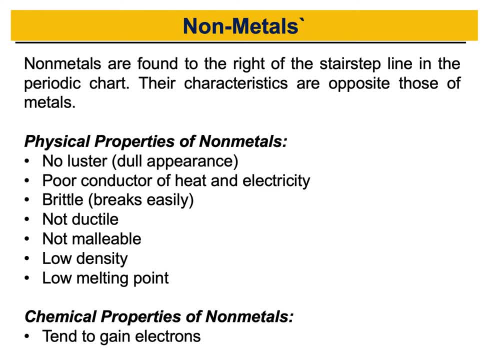 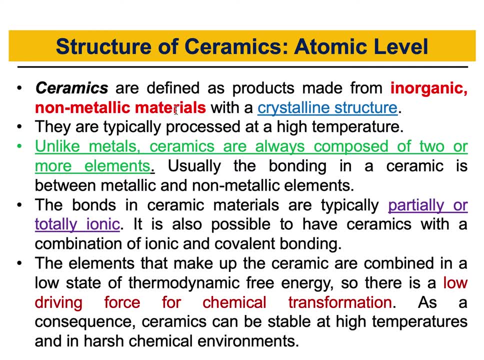 Now, we talked about ceramics before and we said that they are in their properties. We mentioned that they are. you know, they're made of inorganic, non-metallic elements and they are always composed of two or more elements, And we mentioned something about partially or totally. 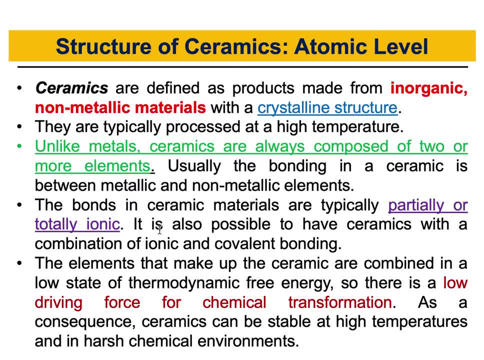 And we mentioned something about partially or totally ionic. It's very important. And if it's not totally ionic, if it's partially ionic, it means that it has also covalent bonding. We need to identify how much of our bonds are ionic, or covalent percentage wise. 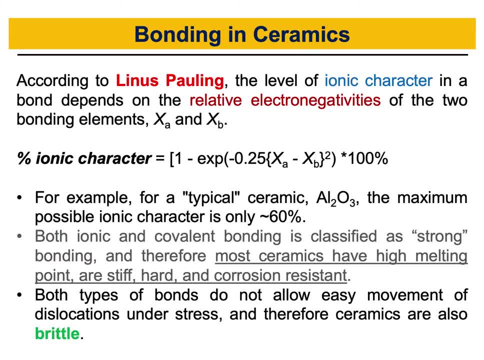 And this brings us to the concept of bonding in ceramics. And according to Linus Pauling, he's a chemist, American chemist. And according to Linus Pauling, he's an American chemist, He's a biochemist and chemical engineer. 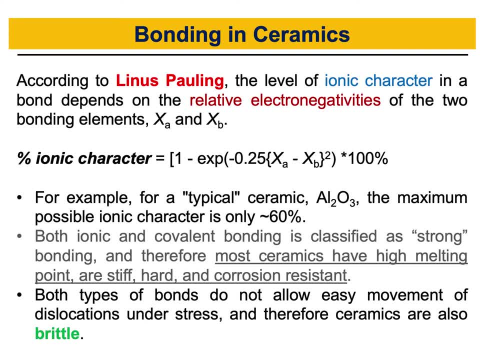 He did a lot of work and research. He published 1,200 papers and books and I think 850, more than 850- of them are scientific topics. So he's a pioneer in chemistry and chemical engineering. So he came up with this concept called the ionic character. 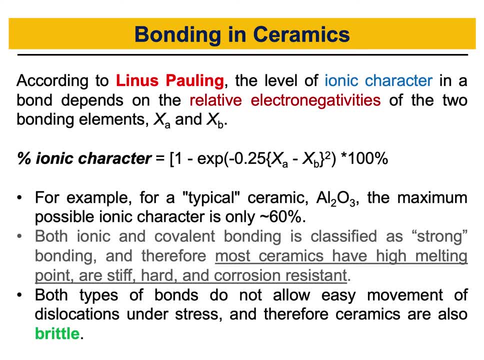 How much of my ceramic is ionic bonding and how much is covalent bonding. And he said that you can characterize the ionic nature of the bond In a ceramic using something called the relative electronegativity. We talked about electronegativity before, so that some elements are more electronegative than other elements. 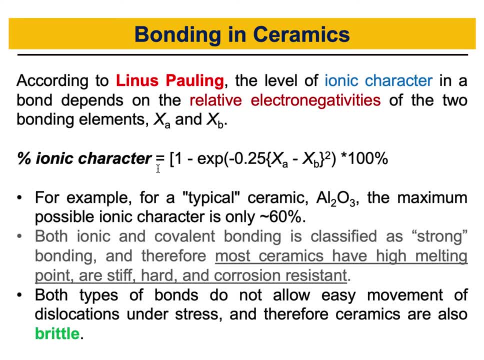 So you can calculate something called the percent ionic character by 1 minus exponential, minus 0.05, multiplied by xA minus xB. These are the A and B are the elements that create my ceramics and the x's are the relative electronegativity. 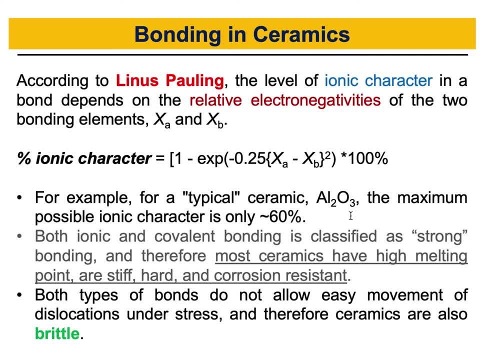 And you can get a number. For example, for typical ceramics, aluminum oxide- the maximum possible ionic character is only 60%. So 60% of the bonds are ionic, while 40% are covalent. in this, Now, there's a lot of it's important and there's a lot of applications, of which one? how much do we need the ionic character to be? 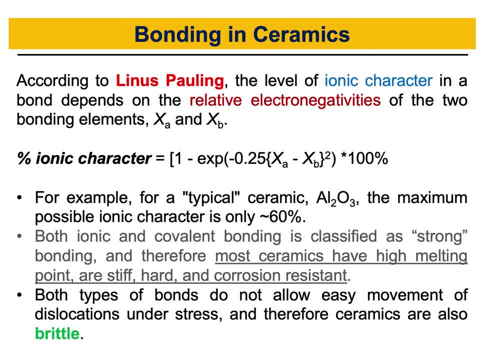 So it's a very important quantity to be identified And if you're Working in your project- I would recommend that you will, If you're working with ceramics- to find your ionic character for the material that you're using. So both ionic and covalent bonding is classified as strong bonds.